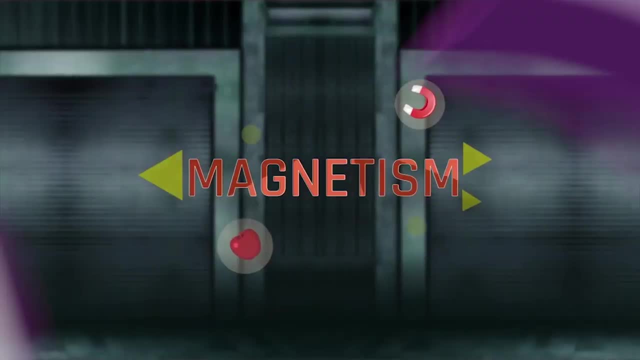 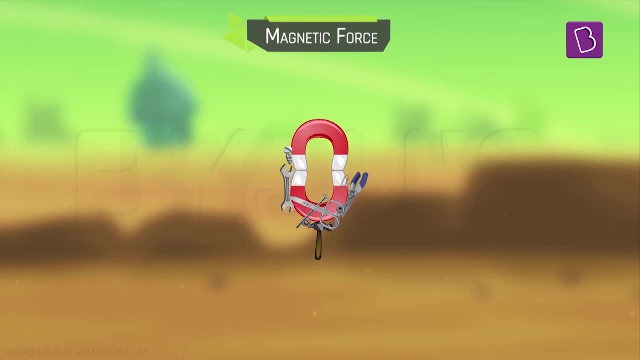 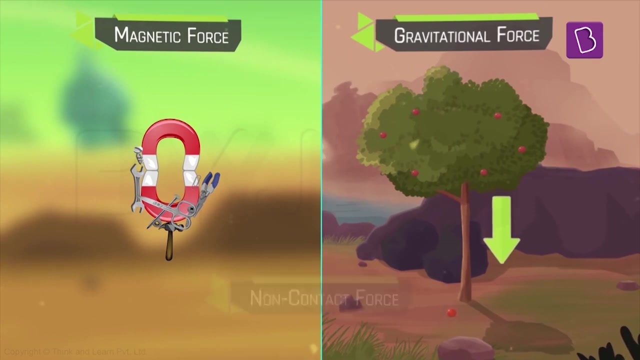 Now, the force that magnets apply on each other and other objects is called the magnetic force and is very similar to gravity in the sense that it's a non-contact force as well. Now, the magnetic force doesn't really require any sort of touching for it to push or pull. 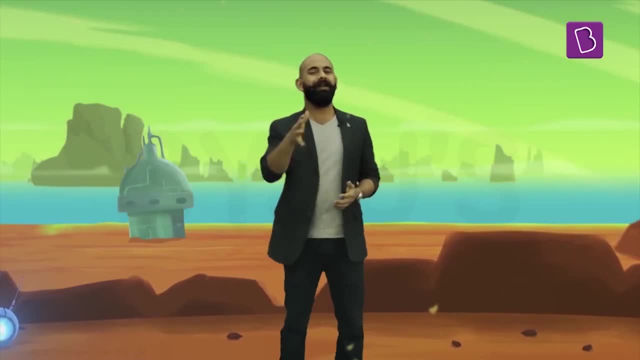 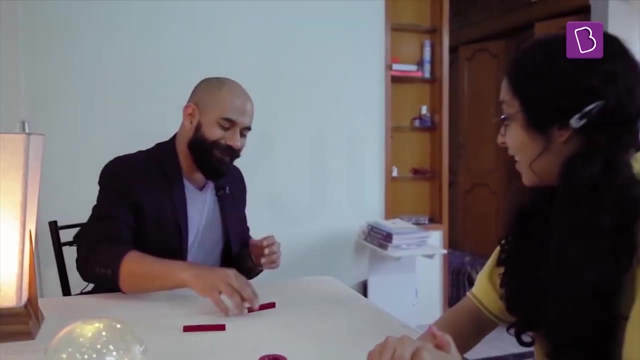 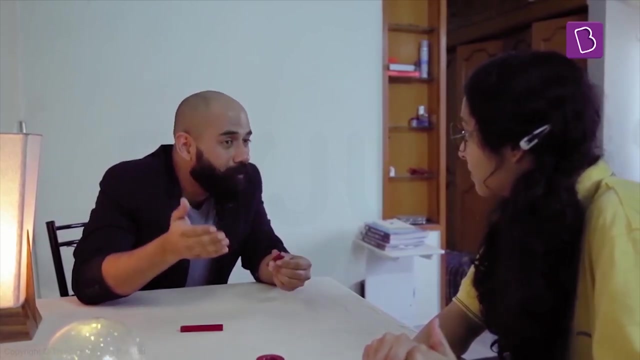 something or affect You know what. let's play with some magnets to see how they work. So this is what you call a bar magnet. Now, any magnet has two sides, which we call poles. It's called the North Pole and the South Pole. Now, if you look at this magnet, the North 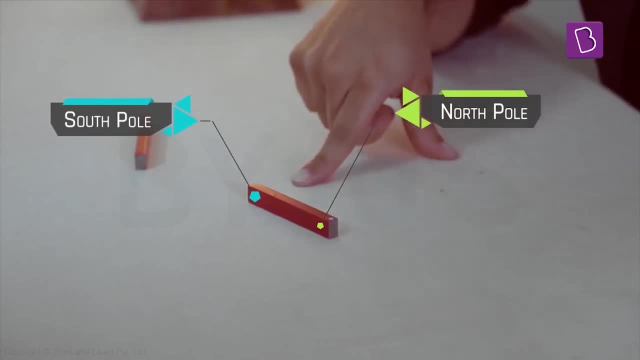 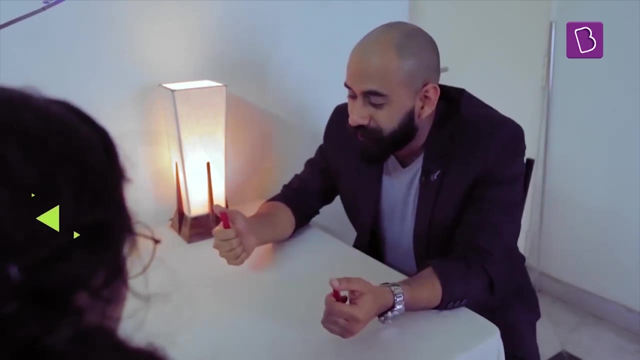 Pole is marked with this white dot. So this is the North Pole and this is the South Pole. Now, when you take two magnets, that's when it becomes fun. For example, what happens is the like poles. they repel each other and unlike poles attract. 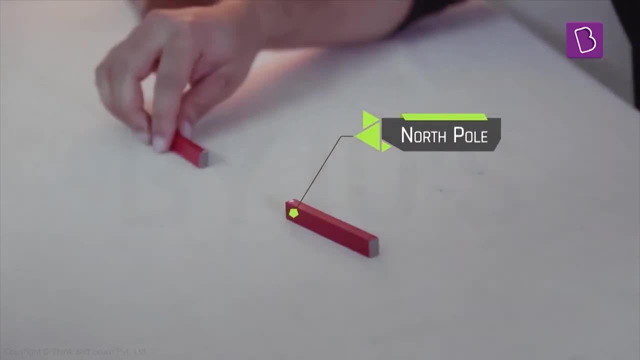 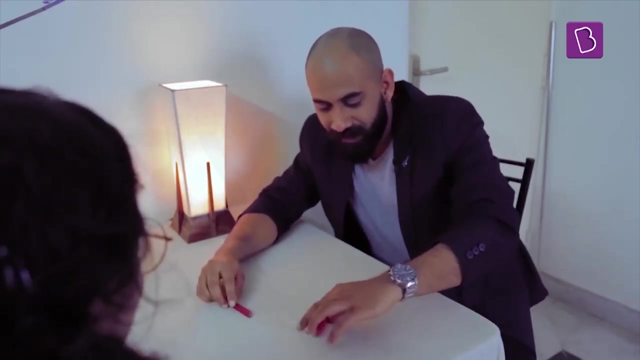 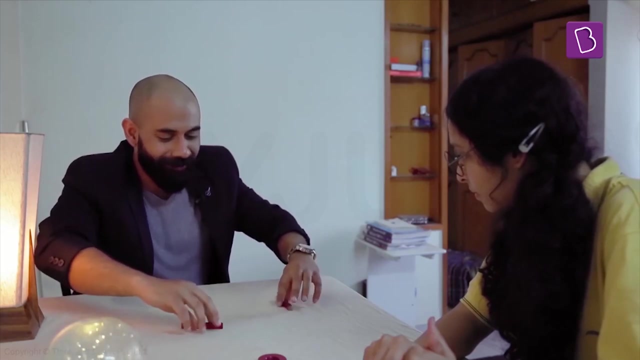 See here, for example. So this is the North Pole and I have a South Pole over here. Look at what happens. You see that, Similarly, if I had a South Pole here and a North Pole here, they attract again. But when we take two like poles, let's say two North Poles, 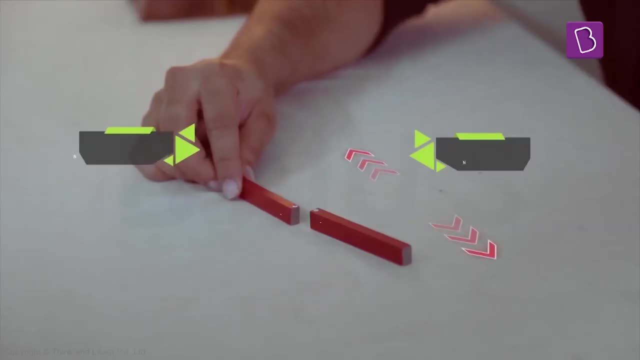 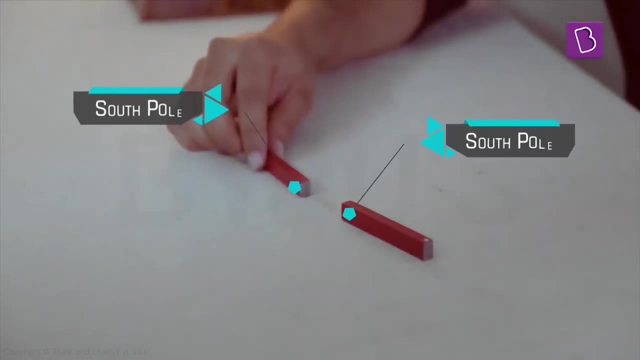 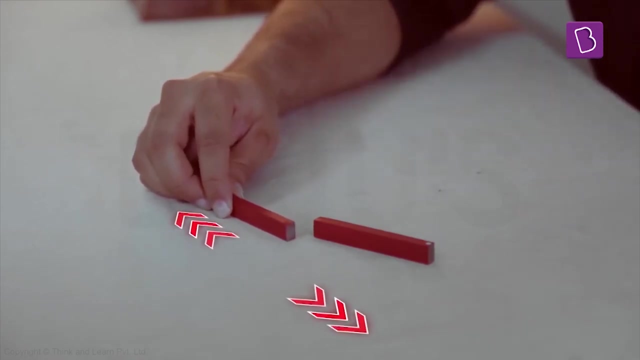 they will. They should repel each other. Yes, like this. See that? And if we had two South Poles facing each other, they will repel again. And the interesting part is that they do this without any sort of contact or touching, which means they are. 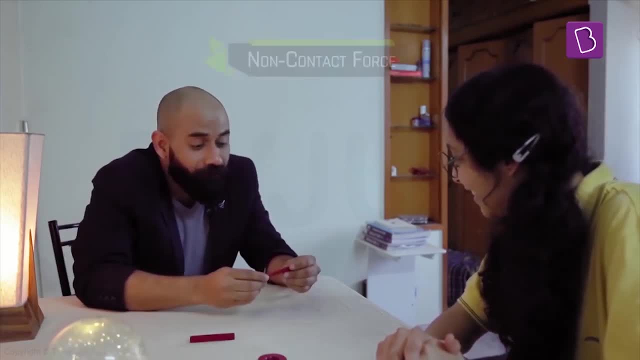 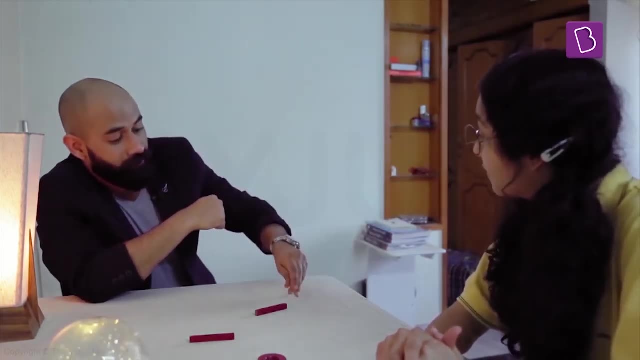 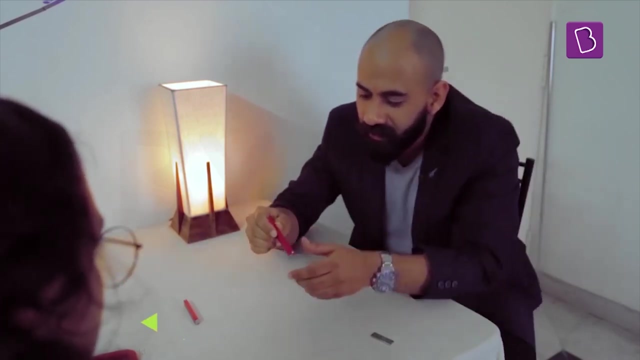 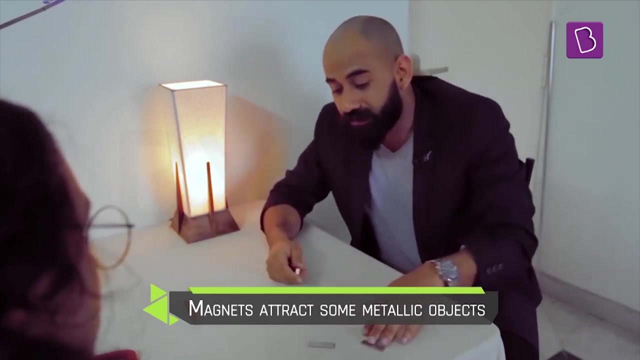 Non-contact forces, Exactly Now. magnets are also fun when you play with metallic objects. So magnets always attract, like certain metallic objects like these. See this. Yeah, Both poles of the magnet attract this object. Of course, magnets don't attract all metallic. 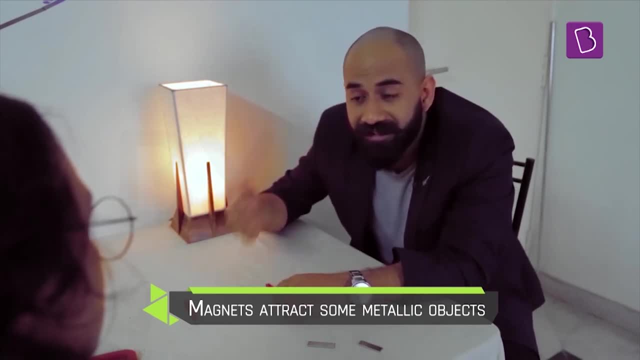 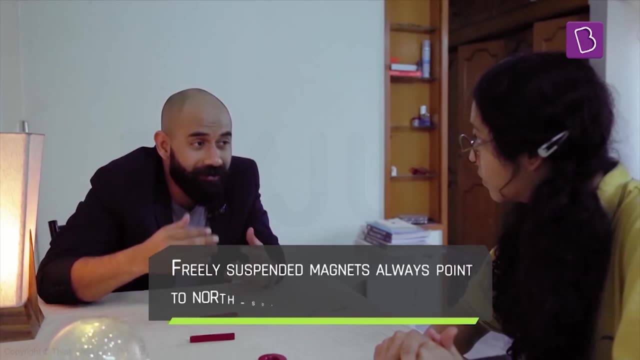 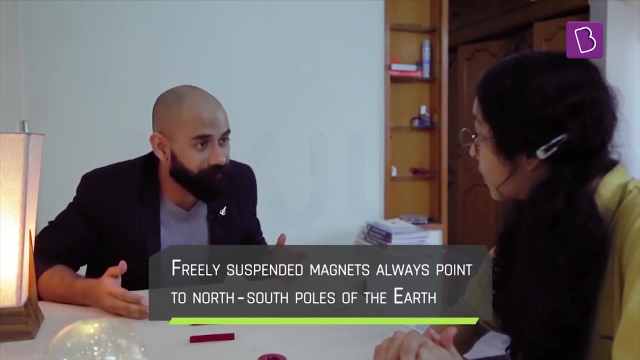 objects. They attract certain kinds of objects like iron and steel. The other interesting thing about magnets is that when you suspend a magnet, it always points to the North Pole. Okay, And this property is used in compasses, So let's say we had a compass.